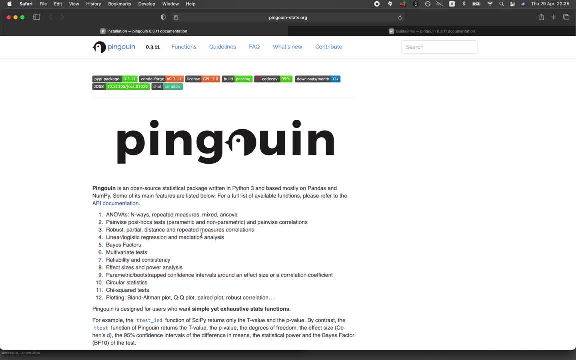 do a long list of statistical analysis, And actually these are only some examples of what it can do, And so for a complete list we have to take a look at the API. And so this Python library is called penguin, And so it is mentioned here that the penguin Python library, when 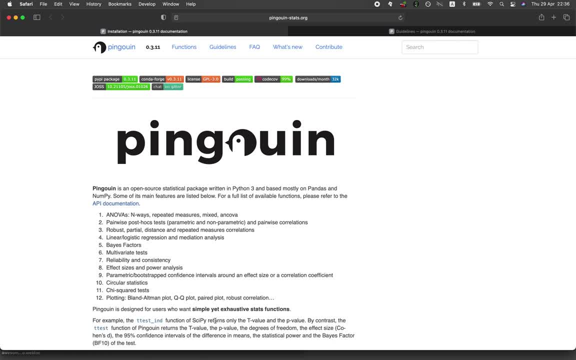 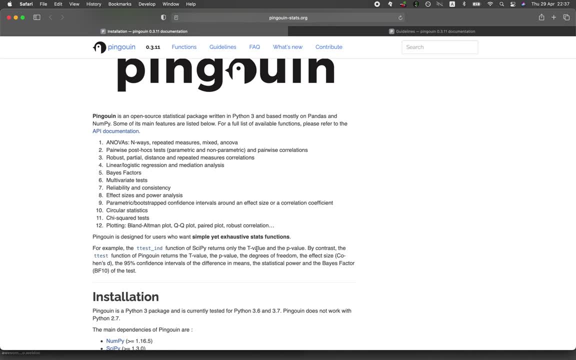 compared to the t test function of scipy, the penguins version of t tests provides more detail, And so you can see that the scipy version provides the t value and the p value, while the penguin version provides t value, p value And, in addition, 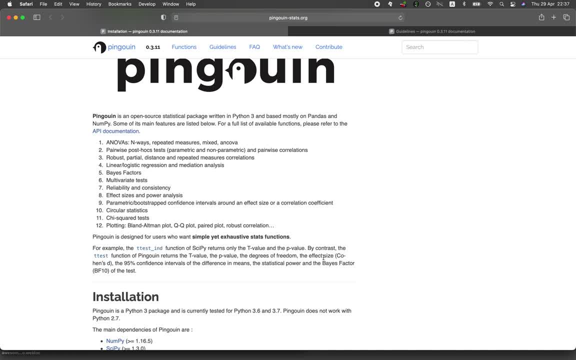 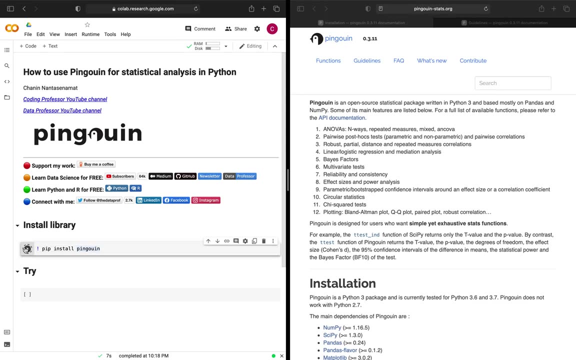 it also provides the degree of freedom, the effect size, the 95% confidence interval of the mean difference, statistical power and also the base factor of the test. And so why don't we get started and install penguin on a Google Colab? So let's install it, pip, install penguin, All right, and 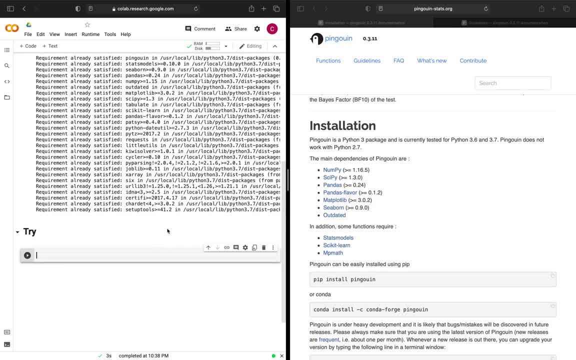 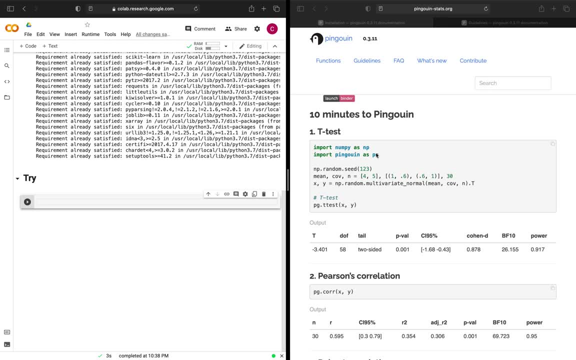 installed already, So actually I've just installed this a few seconds ago, And so that's why it is returning very quickly. And so let's try one of the t tests- Calculation- here. And so on the website of penguin, which you could easily click on this: 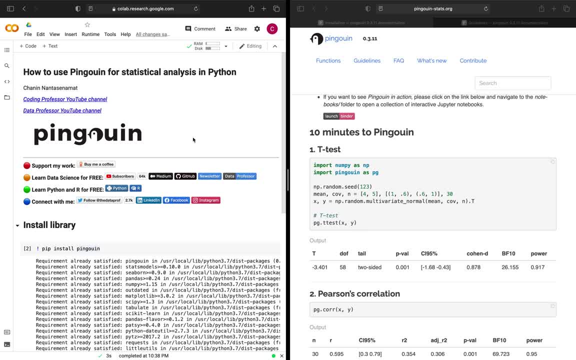 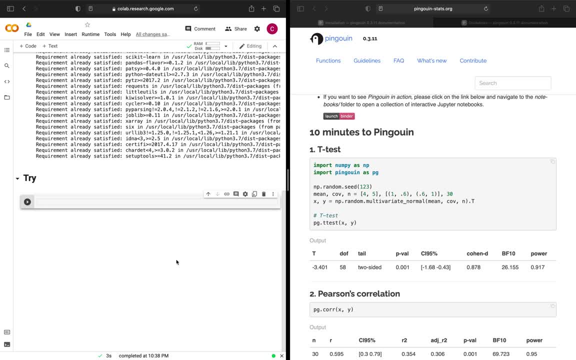 link, And so this particular Jupyter notebook will be shared in the video description, And also I provide the links to this as well in the video description. And so let's try it on Google Colab And so let's do the t test. So first thing is to import NumPy as NP, import penguin as PG. 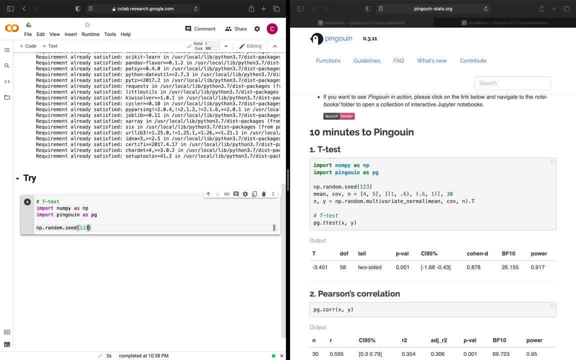 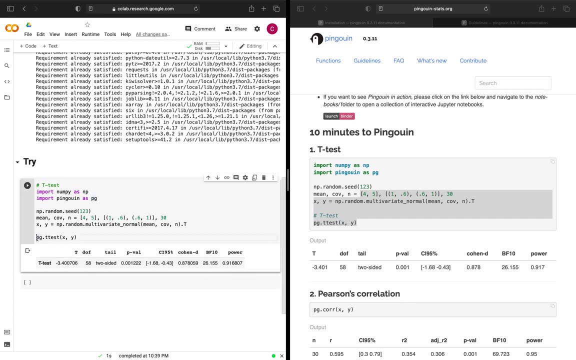 And then we will assign a random seed number in order to allow it to be reproducible. Actually, we just copy and paste the rest. So there you go, it is returned here. So let's say that if we want to put it into a t test, df. 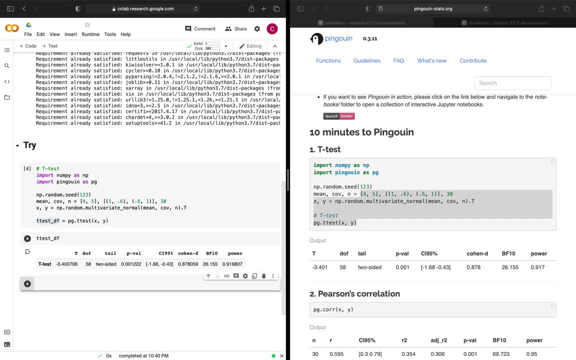 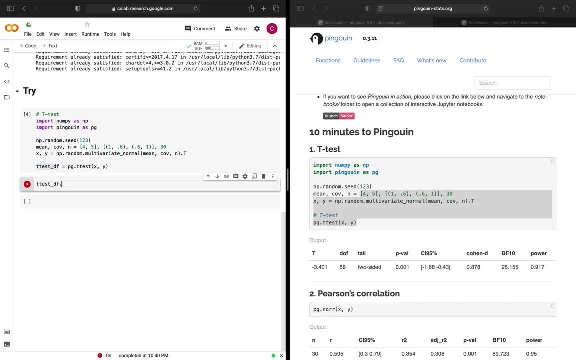 because it looks like a data frame. Let's do that. All right, so it is a data frame. So let's write a CSV file- t test df, dot to CSV- And we'll call it t test dot, CSV. Let's have a look. There you go. 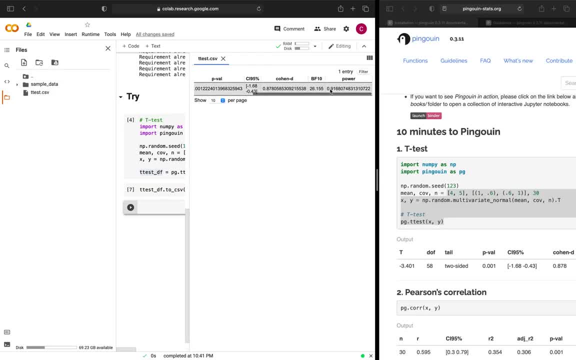 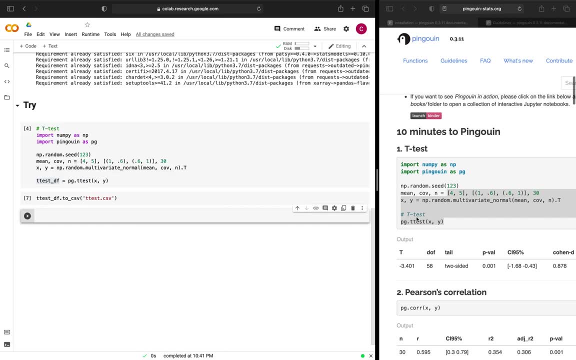 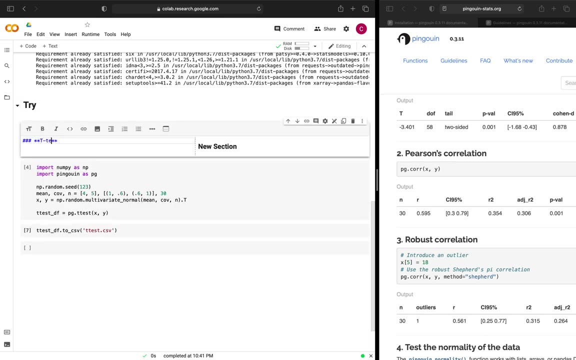 Let's double click on it. Here it is, So it is conveniently printed out, And then we save it as a CSV file. So it is a pandas data frame. Let's try another one. Let's try that Pearson's correlation one. So why don't I make this into a test? t tests. 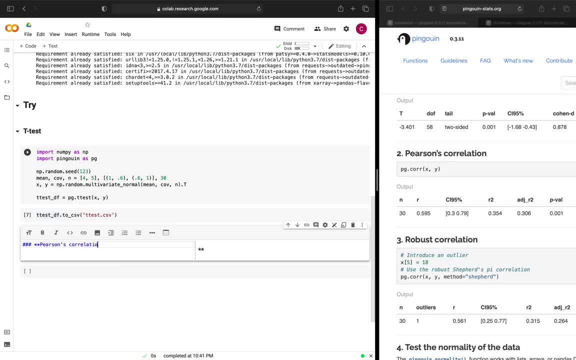 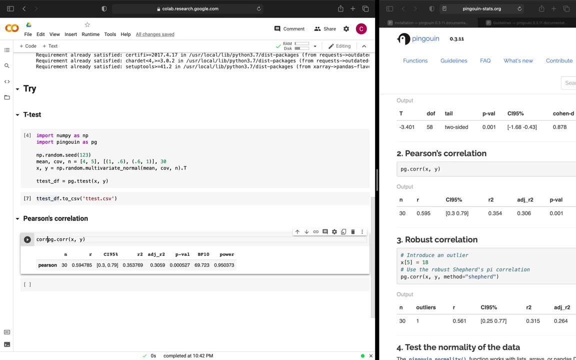 Pearson's Relation. We just need to use PG dot core function, correlation function x and y asked to input arguments, And there you go, And we could assign it to a data frame. Let's call it Z or R, underscore df, And we could also print it out. 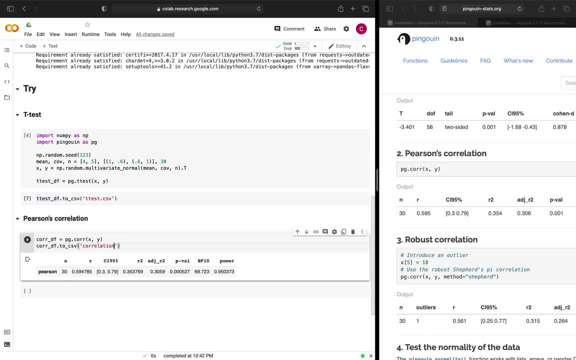 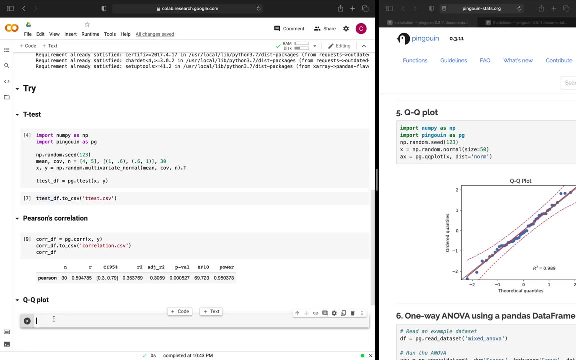 to see this fee because correlation, And then we just return it so that we could see it. There you go. And how about let's have a look at the qqplot here, qqplot, and then just copy it, All right. 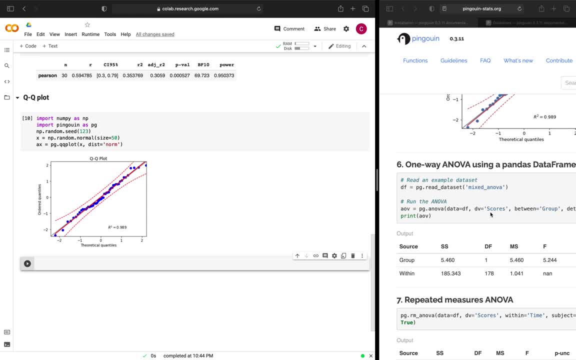 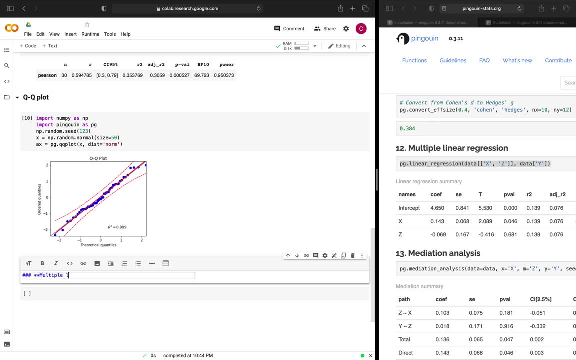 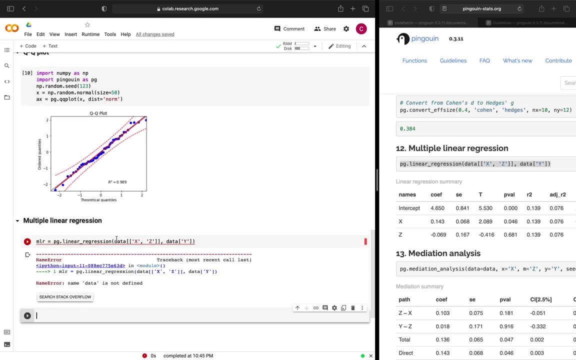 So you could easily generate this qqplot and you could calculate ANOVA. You can perform multiple linear regression. Let's try that QqplotLinearRegression. let's call it NLR. data is not defined. okay, let's see what's. 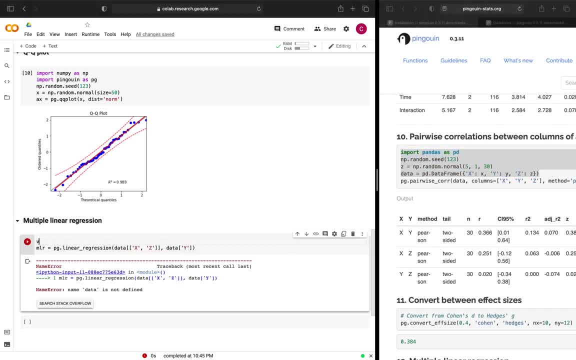 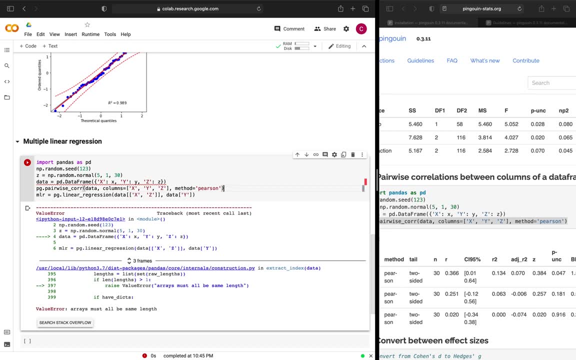 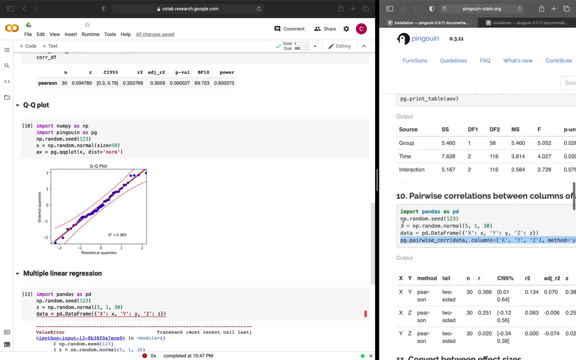 the data here. All right, So we'll use it here. x, y, z. that's why, adding this, that will only calculate the pairwise. We have x here. where did y come from? Z is here. Okay, Let's see define y, because I didn't run all of it. 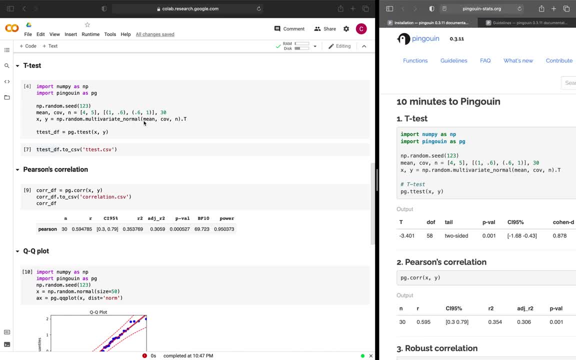 Okay, I didn't find one. Okay, We had y already, x, y, Oh, but it's for the t-test example. Let's search for y, Let's run this again And then let's run that, Oh, okay. 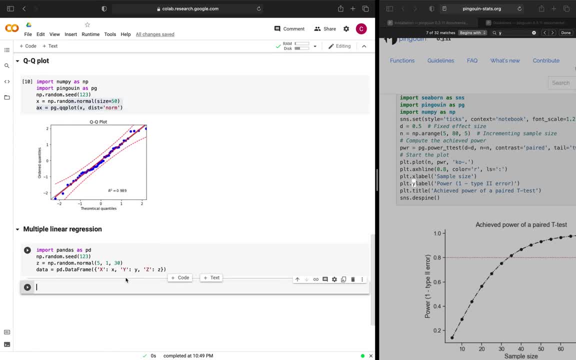 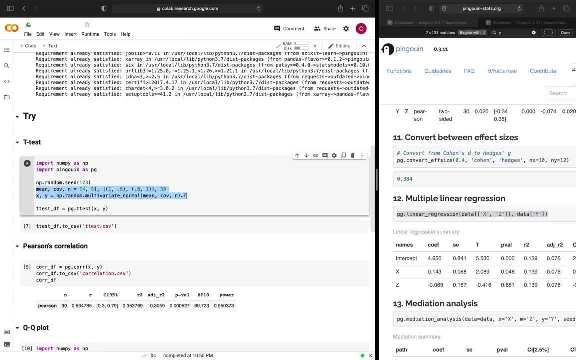 Maybe it works. Let's try. Okay, It works. now Let's put that here. Let's reuse the chunk of code here and let's put it here. There you go. Okay, Let's see, Let's see, Let's see. 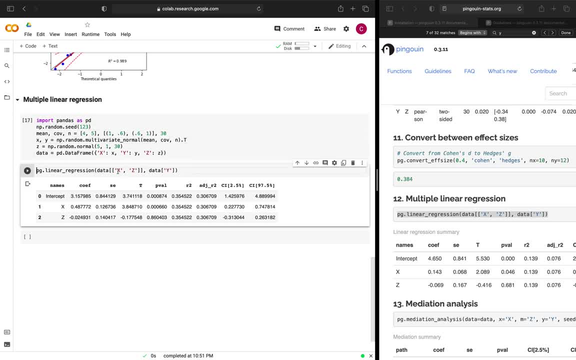 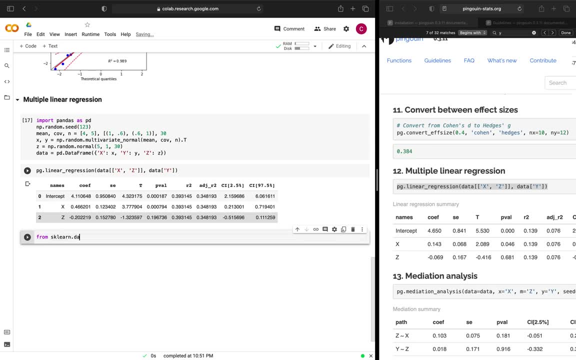 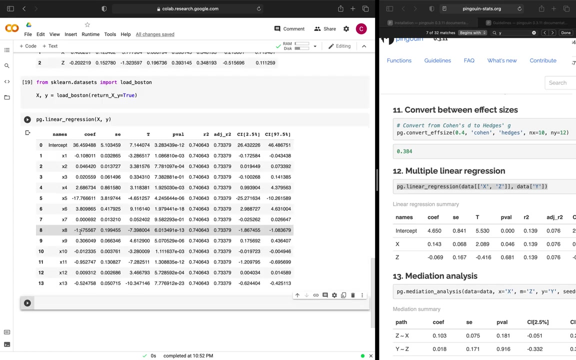 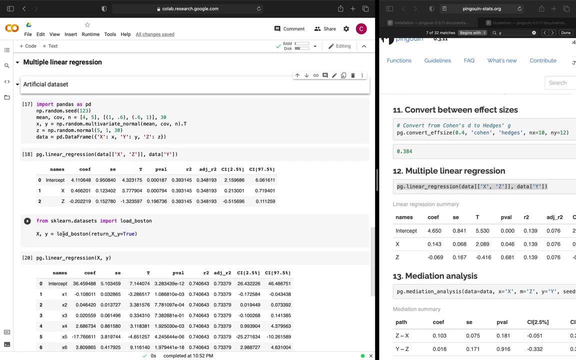 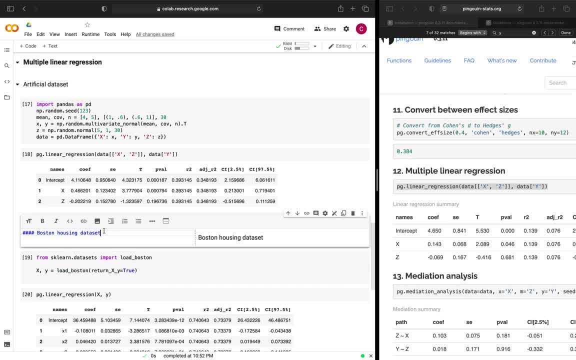 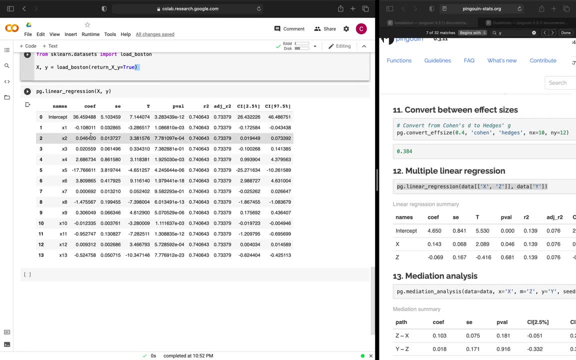 Boston, Kelsey data sets. Let's make it bold. All right, there you go. And now you can see the coefficients, the regression coefficients of all of the independent variables and the intercept value as well. All right, here we go. 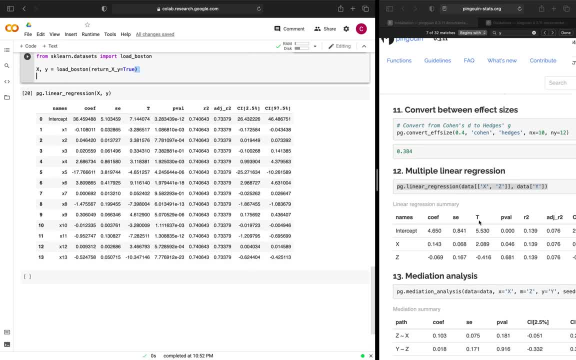 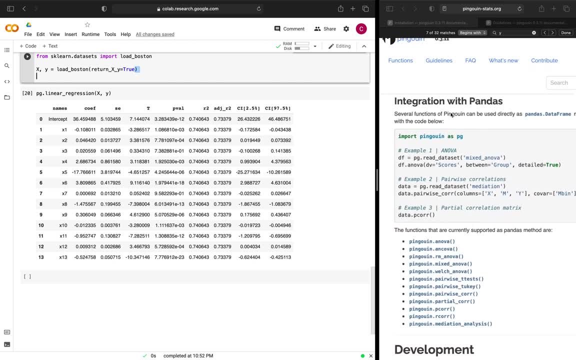 The R squared value, the adjusted R squared value. All right, so let's continue And let's have a look at this feature here. So it's so. it is saying that penguin is integrated with past and future. So it's saying that penguin is integrated with past and future. 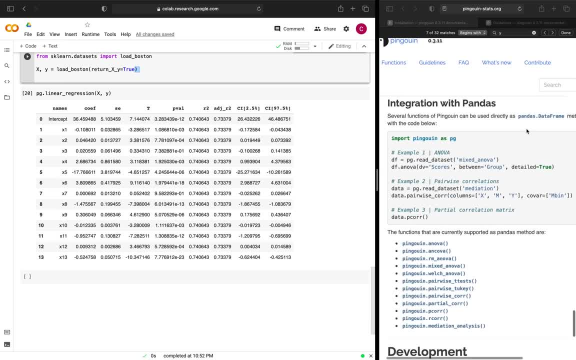 So it's saying that penguin is integrated with past and future, integrated with pandas data frame, And so you could add a function after the data frame itself. But then apparently here they're reading in a data sets from the penguins library. 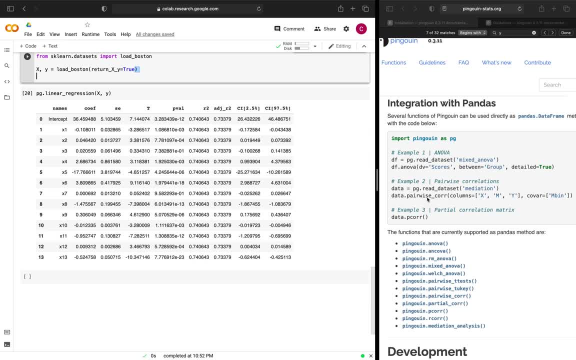 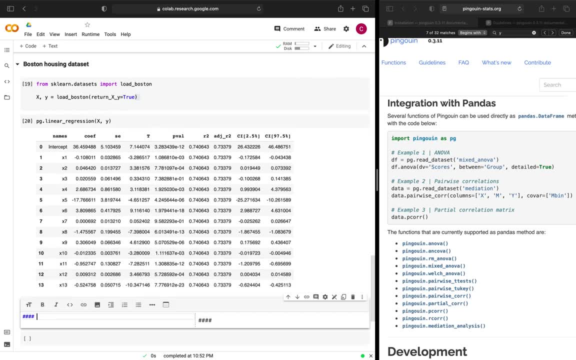 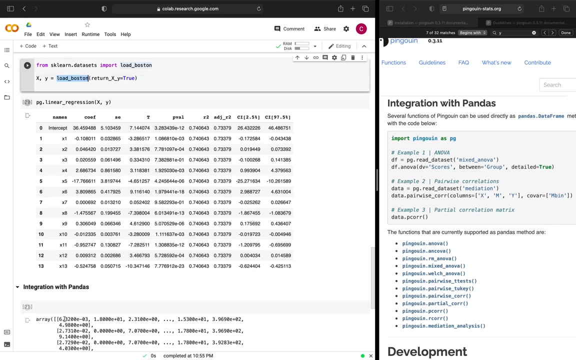 So I would imagine that if we apply the functions here on a pandas data frame, I think it would work. Let's see, Let's improvise here Integration with pandas. Oops, And let's see, We have our XY. It's not yet a pandas data frame here, Load Boston, Okay, So let's create our own. 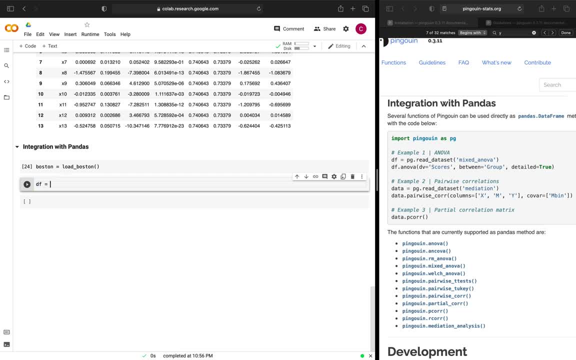 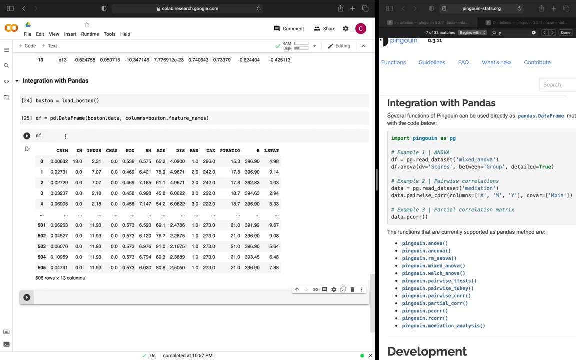 Let's call this Boston. Let's create a data frame, So PDE data frame. We'll have Bostondata columns equals Bostonfeature names. Let's see. All right, So now we have all of the X variables here And let's integrate the Y value. I mean the Y variable here. 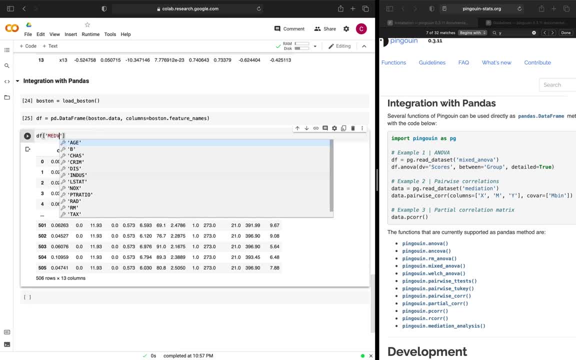 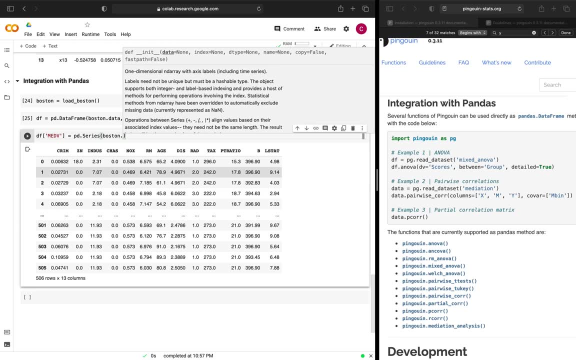 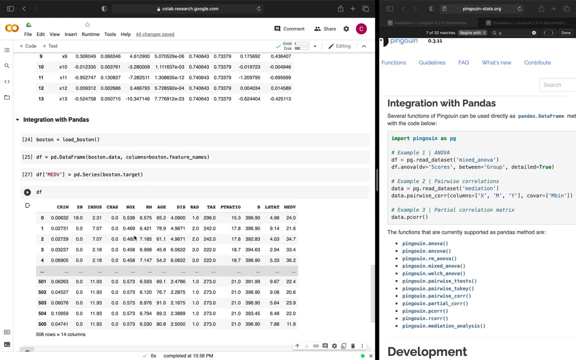 And it's net V. I guess Let's call it. net V equals PDEseries, Bostontarget. Let's have a look again. And now the Y value, I mean the Y variable, is here Net V, the median price of the house. And now it is a data frame, And let me apply the pairwise. 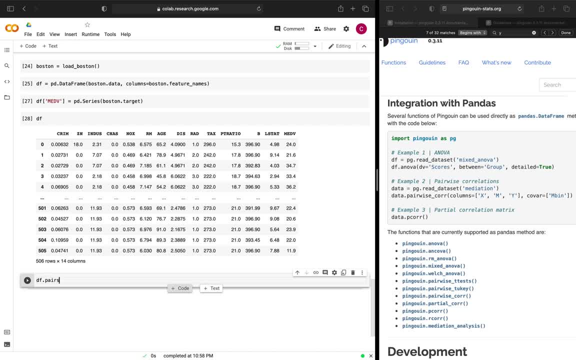 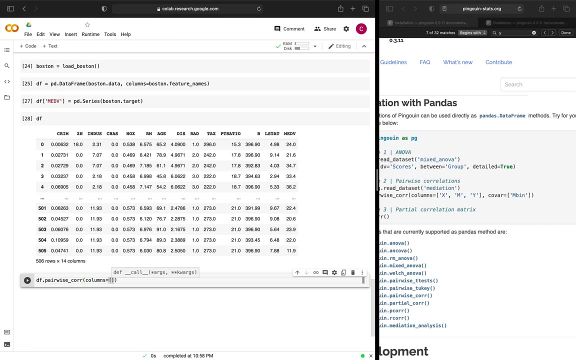 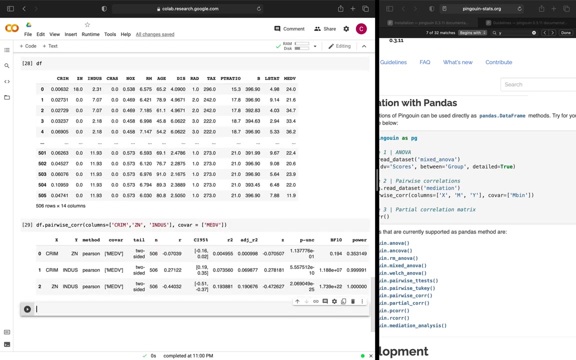 correlations: dfpairwise columns equals, And then we probably have to specify the columns that we want to compute the. So before doing that, let me try columnscrim and zn and endus comma, col- good news. And then net V. All right, 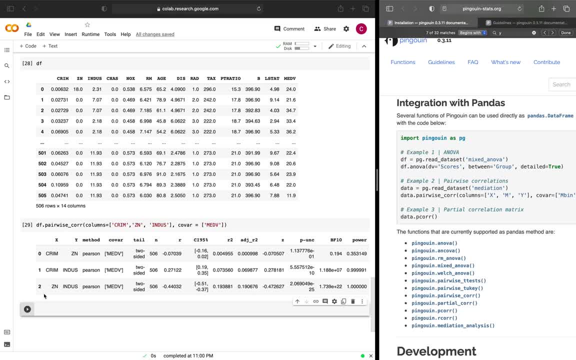 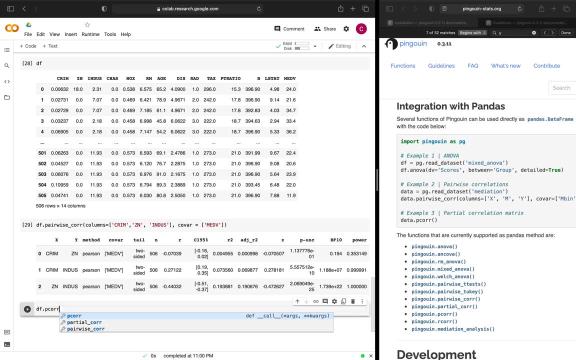 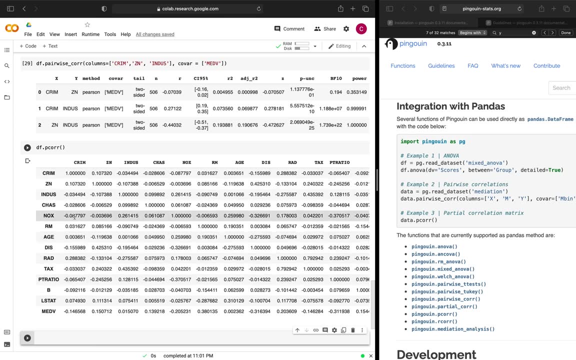 There you go. Okay, So it's computing in all possible pairs for the three. Let's try it on partial correlation matrix. All right, So that was quite easy. So here we have the inter-correlation matrix between each of the variables with one another. 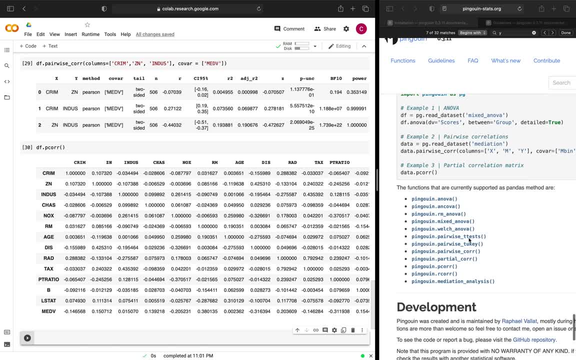 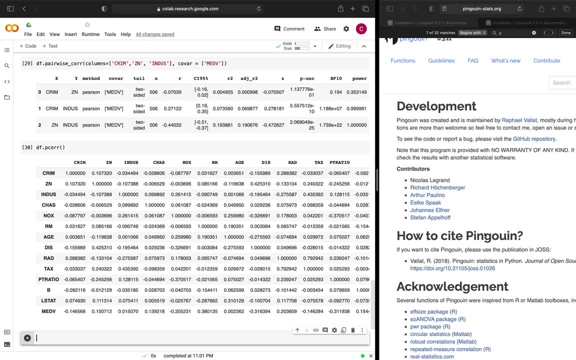 And the correlation with itself will have a value of one. All right, So it works with the pandas data frame, And if you're using this in a scientific paper, then you're recommended to cite Penguin by citing this article. So you can see here that it's quite intuitive. 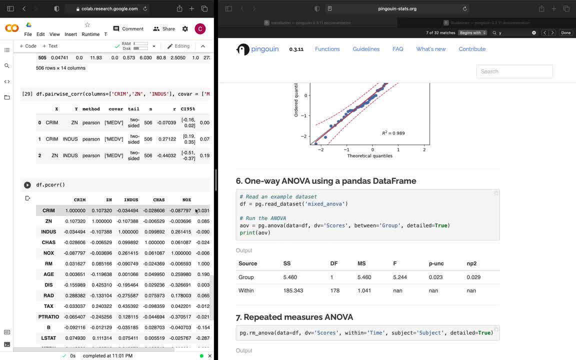 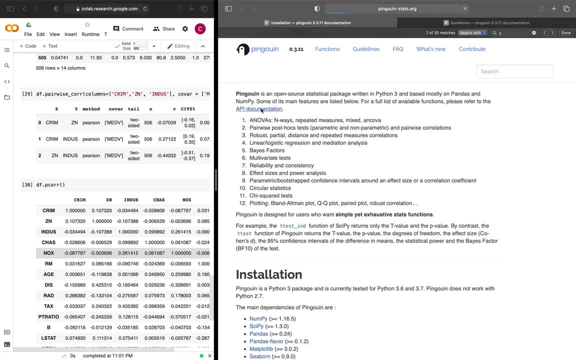 and you could go along by having a look at the example and then improvising in your own projects, But also you could check out the API. You could check out the API. You could check out the API as well. Click on the API documentation And then for all of the statistical 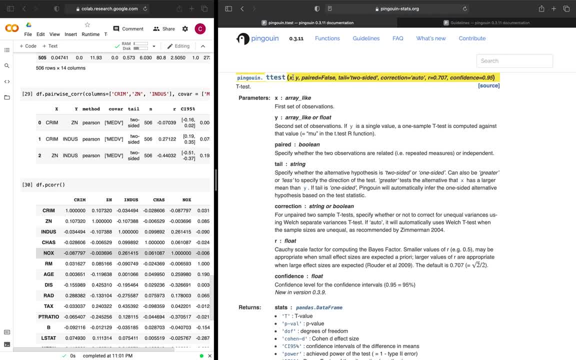 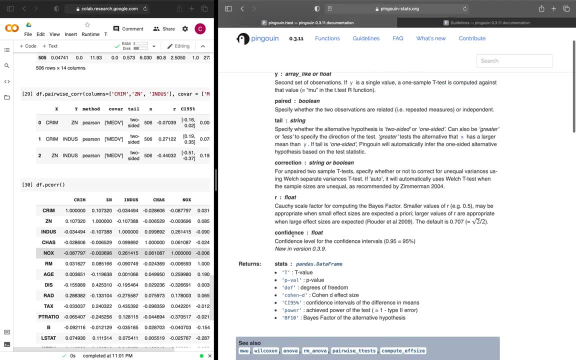 analysis. you could click on the particular function that you want to use and then have a look at each of the import argument and what are the options available for you, And it provides you quite a detailed explanation, and it's good that they also provide some. 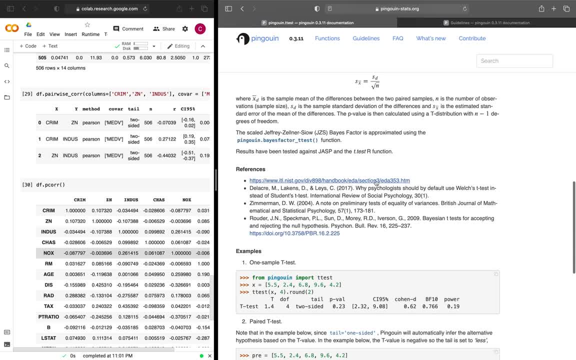 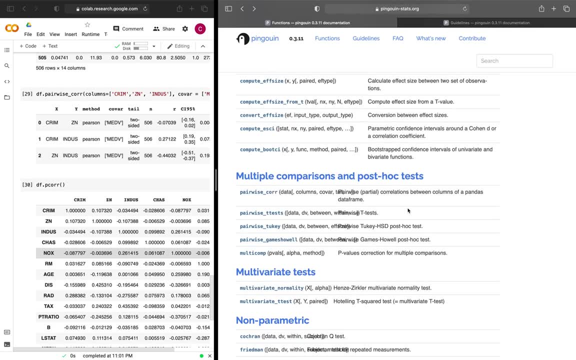 relevant information and also references for you to have a look, and also some more examples we used to try. Let's go back. Okay, So there is a lot of data. Okay, So there is a lot of data. Okay, So there is a lot of data. Okay, So there is a lot of. 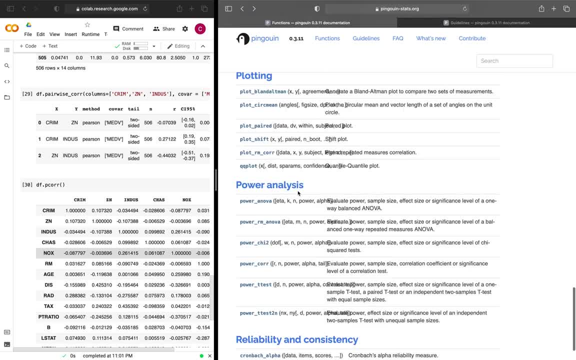 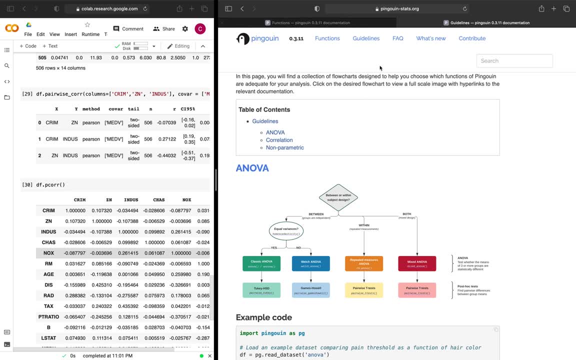 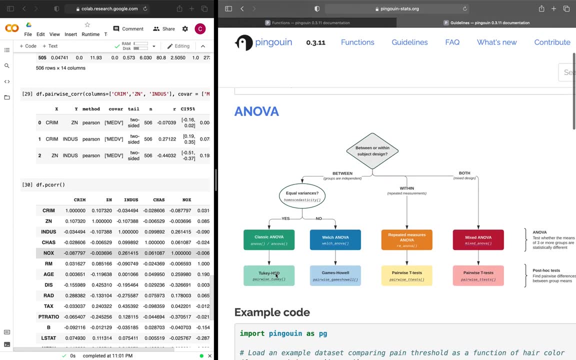 statistical analysis functions available here, And lots of plots as well. Let's have a look at this guidelines. So, in performing statistical analysis, this particular guideline comes in handy because it provides you with a schematic diagram that helps you to select the appropriate analysis for each of the given situation. So they provide you with this decision diagram. 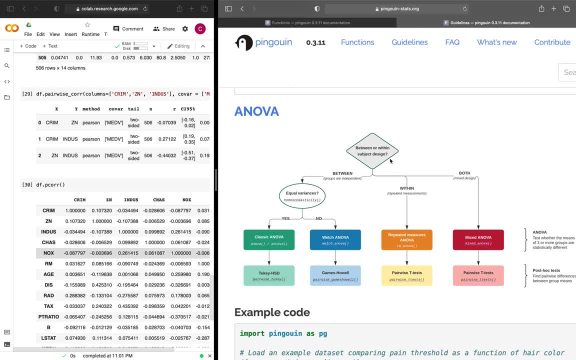 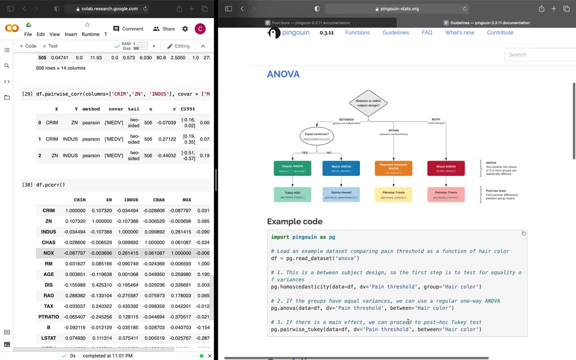 whether you're using between or within subject design or both, And so it will pinpoint you into determining whether it has equal variances, and if it does or if it doesn't, which approach should you use in all of the following functions here? And then they provide you some example code. 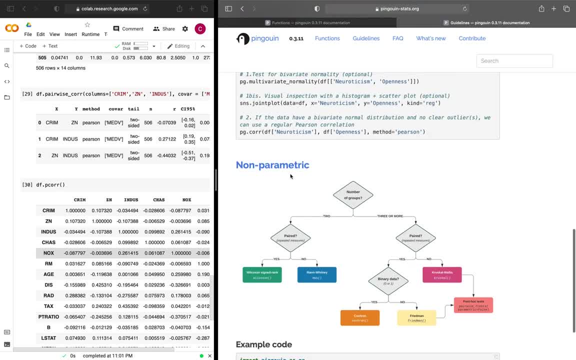 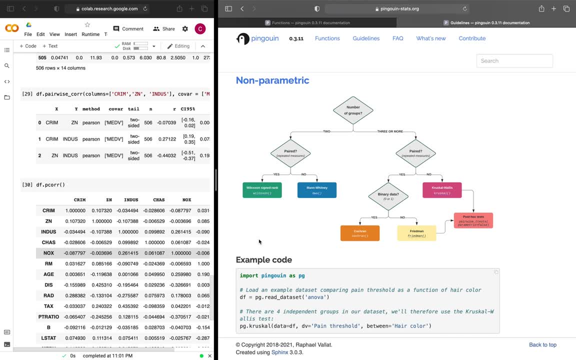 and this is for correlation and this is for non-parametric analysis, And so these come in handy. So I'll provide you the link to this particular page And so, if you're finding value in this video, please support the channel by smashing the like button, subscribing, if you. 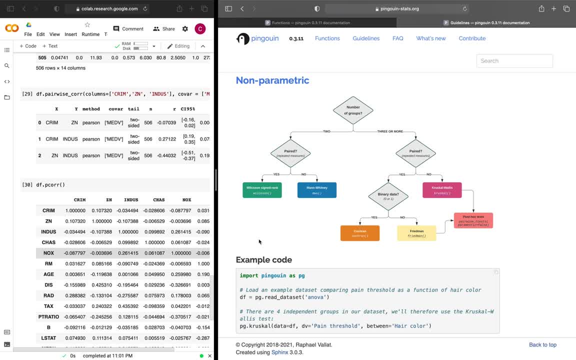 haven't already, and also make sure to hit on the notification bell so that you will be notified of the next video. And, as always, the best way to learn data science is to do data science, and please enjoy the journey. 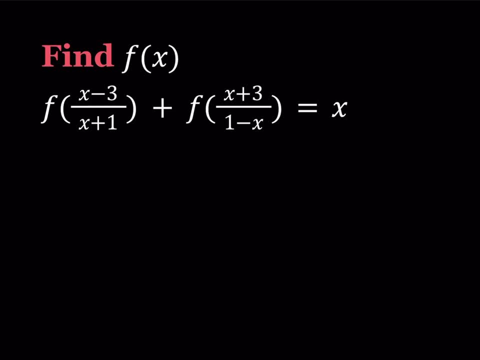 Hello everyone. In this video we're going to be solving a functional equation from the book Putnam and Beyond. I already told you about the book in another video. I'll also share some links down below. Let's get started. So we have the equation f of x minus 3 over x plus 1 plus f of 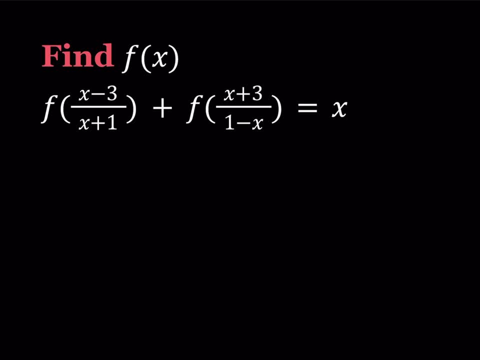 x plus 3 over 1 minus x is equal to x and we're supposed to find f of x. Obviously, we have certain conditions here. For example, x cannot equal negative 1 and x cannot equal positive 1 either. Now I'm going to use substitution, Needless to say right, that's my one of my favorite methods. So